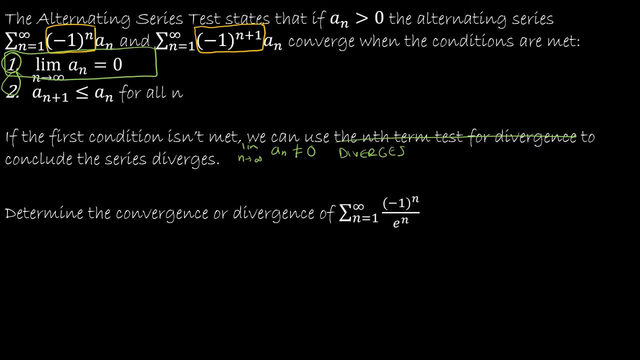 can just say it diverges using the nth term test for divergence. So let's take a look at our first example. We have the summation as n goes from 1 to infinity of negative, 1 to the n over e to the n. Remember that we have to check each. 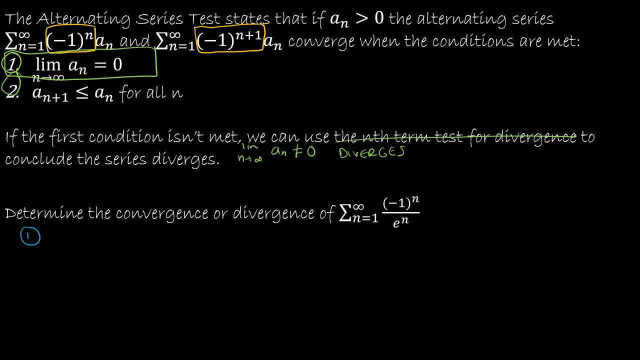 condition. So, for example, if we take 2 points and the sum in the room, we don't have any. So we're going to check condition one and we're going to say the limit as n approaches infinity, of a to the n. 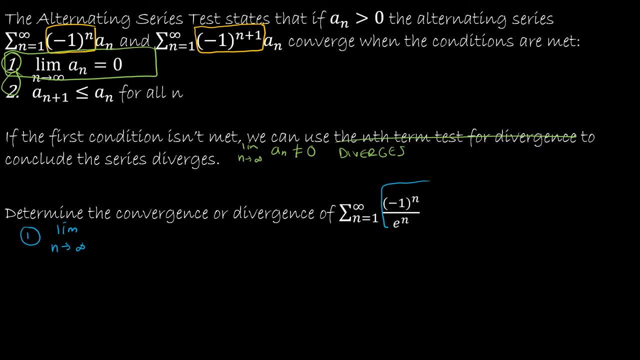 So what is a to the n? When we're looking at this function, we want to really take out the negative one to the n. We want to take out the alternating part. So we're going to let a sub n. I think I said a to the n, but you understand, I meant a sub n. 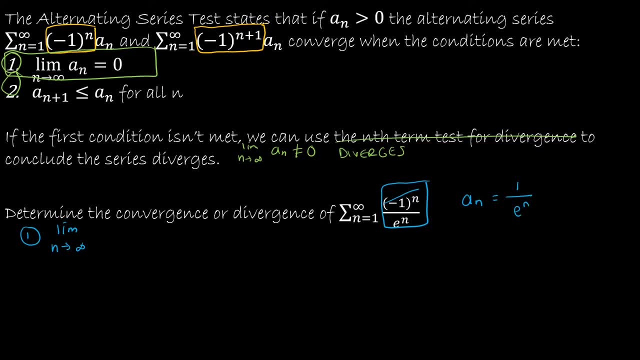 We're going to let a sub n be one over e to the n, Because we're not going to worry about whenever we have the alternating part. we're going to take that out of the equation. So I want the limit, as n approaches infinity, of one over e to the n. 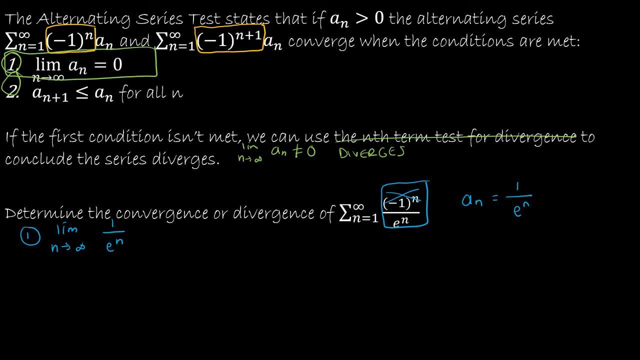 Now what is that limit? As n increases, the denominator is going to get increasingly large and therefore the value of the fraction is going to get increasingly small and approach zero. So the first condition is met. The second condition says that we need to verify that a sub n plus one is less than or equal to a sub n for all n's. 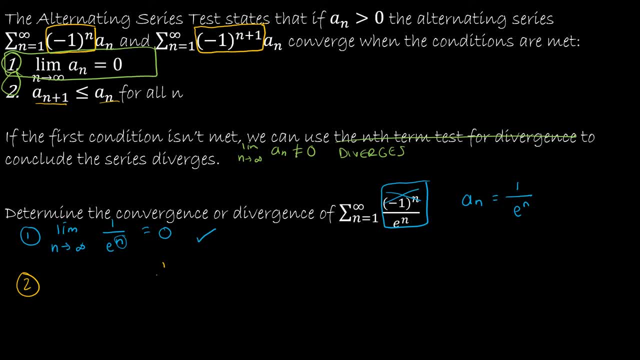 So if a sub n is one over e to the n, as we set up here, a sub n plus one is one. well, let's write it this way: a sub n plus one Would be equal to one over e to the n plus one. 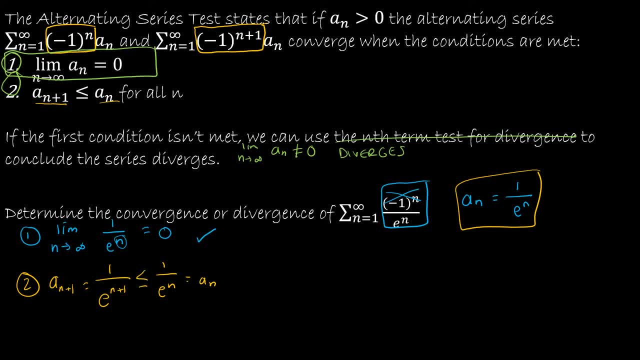 So my question is: is this correct? Can I correctly say that one over e sub n plus one or e to the n plus one is less than one over e to the n? And I can, So you can just reason through it and say: okay, well, this guy is going to be bigger and therefore the whole fraction will be smaller. 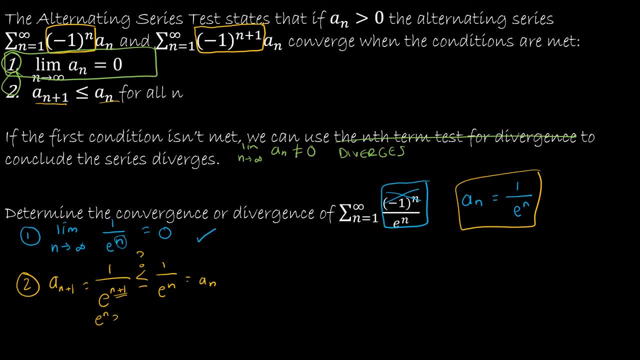 Or you can say: hey, this is like e to the n And e to the first, And obviously that makes this denominator bigger and therefore the whole fraction is smaller. So essentially, I have now checked both conditions And they're both met. 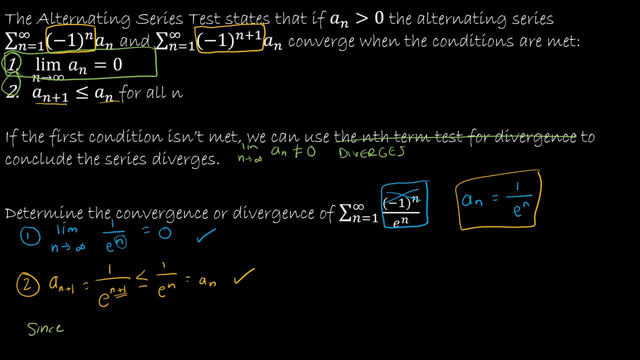 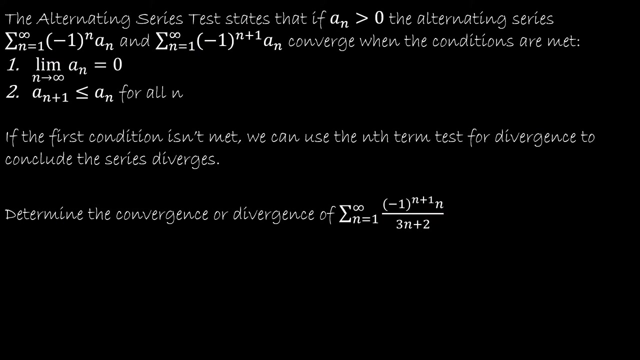 And so I can say, since both conditions are satisfied, Okay, The summation, as n goes from one to infinity of negative, one to the n, over e to the n, converges by the alternating series test. Let's take a look at another example. 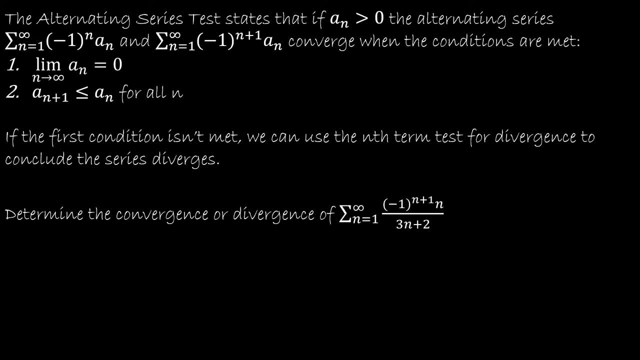 Again. I've left all of the information on the screen so that you don't have to look back and try to memorize what the alternating series test said. So we're going to look at the summation as n goes from one to infinity. 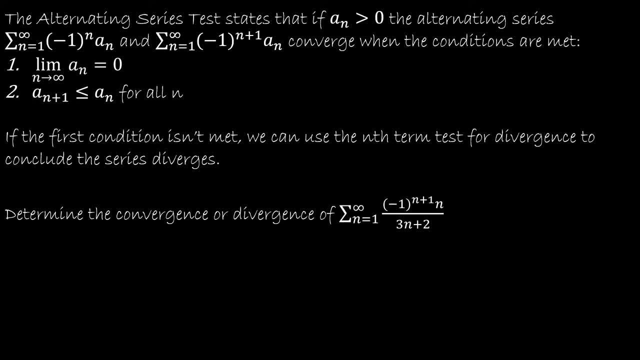 Of negative one to the n plus one times n over three n plus two. So the first thing I need to do is think about what's a sub n. And a sub n is when I essentially take out the alternating part of the series. So a sub n is just n over three n plus two. 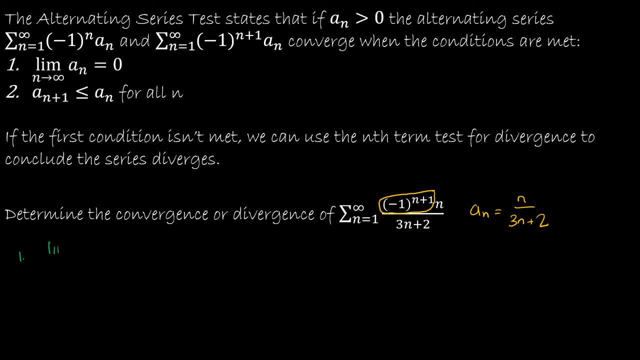 So now I'm going to take a look at the limit, as n approaches infinity, of n over three n plus two. So as n approaches infinity- remember I'm looking at these influential terms. So what I'm going to end up with is the same thing as the limit as n approaches infinity of n over three n, which, of course, is just one third. 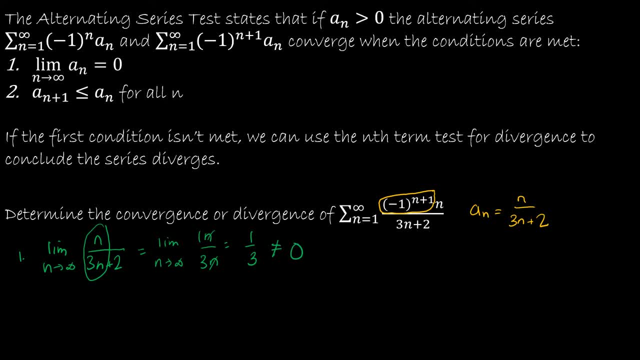 This does not equal zero, And so, again, if the first condition isn't met, we're going to use the nth term test for divergence. to conclude, the series diverges. So I'm going to take a look at the first condition And so, again, if the first condition isn't met, we're going to use the nth term test for divergence. to conclude, the series diverges. 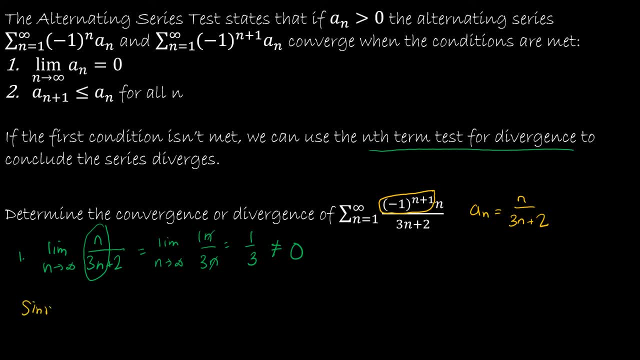 So I'm going to say, since the limit, as n approaches infinity, of a sub n does not equal zero, then the series diverges by the nth term test. And so, again, if the first condition isn't met, we're going to use the nth term test for divergence. to conclude, the series diverges. 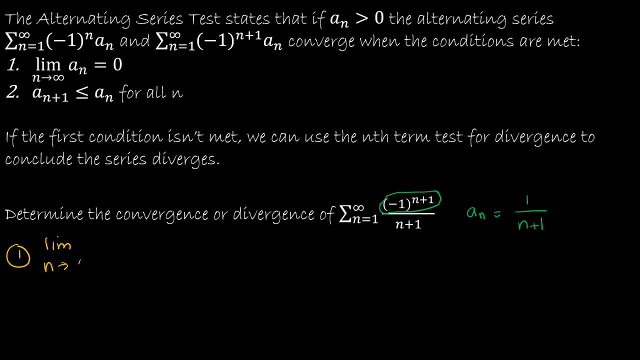 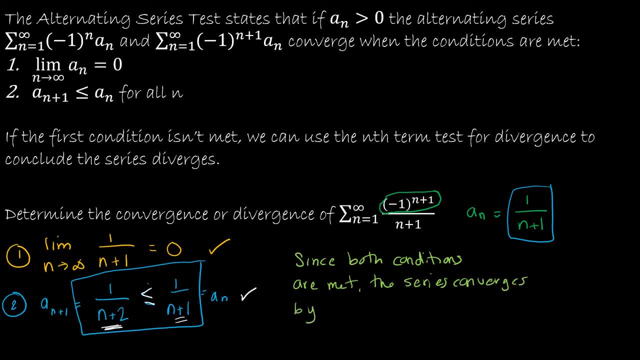 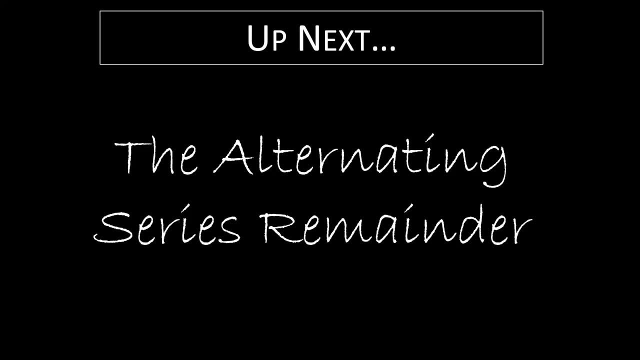 And so again, if the first condition isn't met, we're going to use the nth term test By the alternating series test Up next, we're going to take a look at the alternating series remainder, which is not a test, But, if you'll recall, we have always been asking two questions. 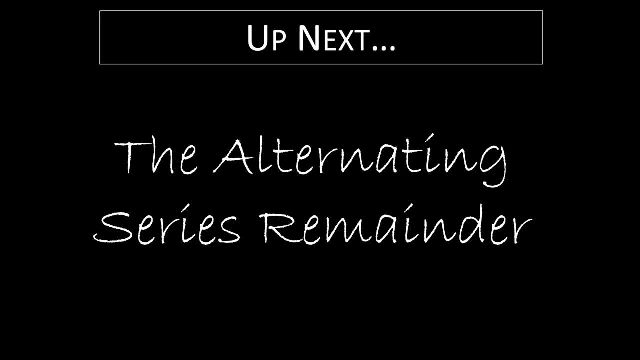 Does the series converge or diverge? And if it converges, what is the sum? So we haven't really been looking at the sum, And so the alternating series remainder is going to help us come up with an estimate of the sum. And so the alternating series remainder is going to help us come up with an estimate of the sum.